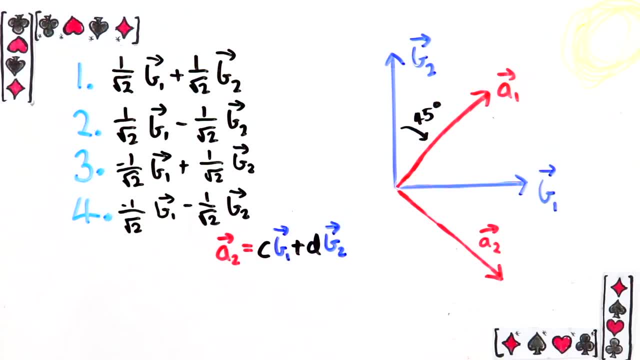 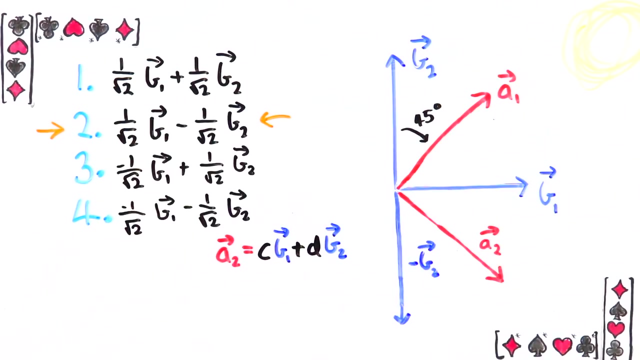 you should be able to work it out from where the minus signs are. Pause the video now to think about it. The answer is 2.. b1 minus b2, divided by square root 2.. This is because if you turn b2 around to get minus b2, then add these two vectors. 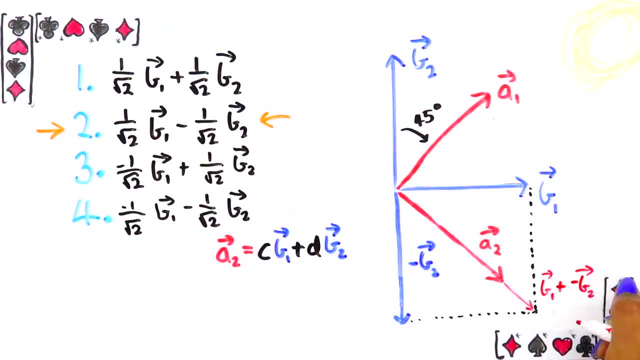 you do get something in the same direction as a2, but it needs to be shortened. If you weren't sure how to approach that question, may I suggest my video on vectors as a reference. The link is in the description and in the corner. 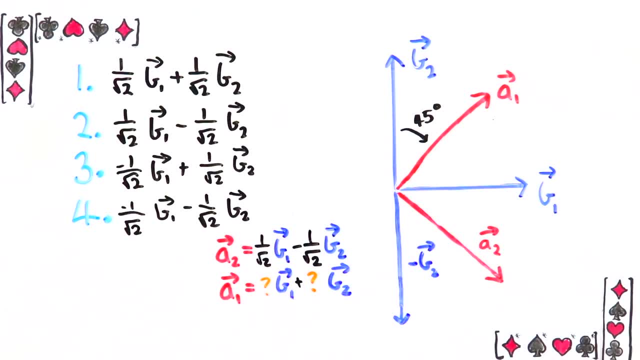 Now say that Alice wanted to write her first basis vector in Bob's basis. Which one of these options would that be? Hopefully you can see that it's 1.. Okay, so Alice now knows how to write these two basis vectors in Bob's language. 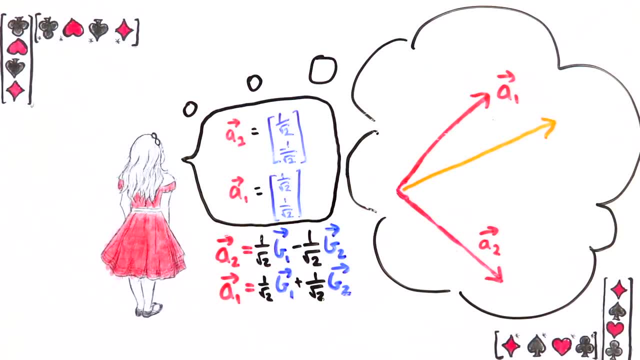 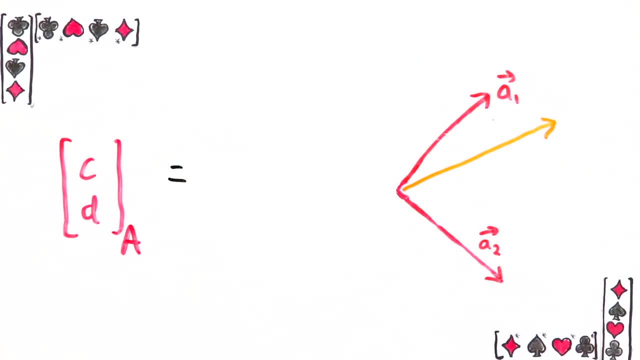 But what if she wants to send some other vector? Well, now she basically can. Why Imagine she writes her vector as this column of numbers. That means the vector is this linear combination of her basis vectors. She needs to translate this whole thing to Bob's basis. 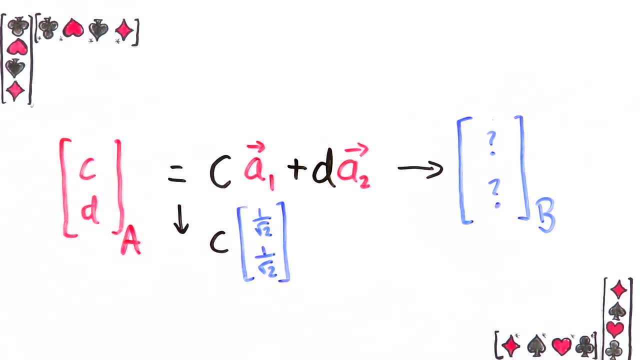 But she already knows how to translate her own basis vectors, And after doing that, she's done right, Because the resulting column is in Bob's basis. Now Alice can write her own basis. now What we've learnt from this example is: no matter what kind of vector Alice has, 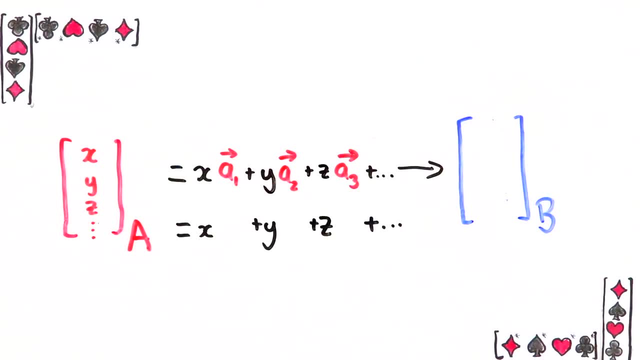 and what basis she's written it in. as long as Alice somehow figures out how to write each one of her basis vectors in Bob's basis, that's enough to translate her vector to his basis. We could leave this here and be happy, but there's a really convenient way for Alice to do all this translating. 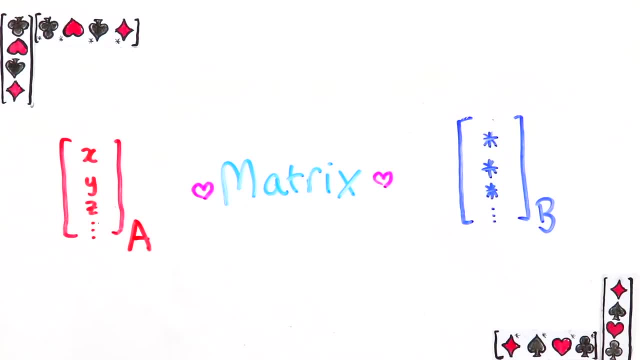 We could represent it as a matrix, As in: Alice just puts in her vector in her basis and the matrix spits out what it should be in Bob's. We're going to call this the change of basis matrix. Going back to our example, Alice knows that her first basis vector is written like this: 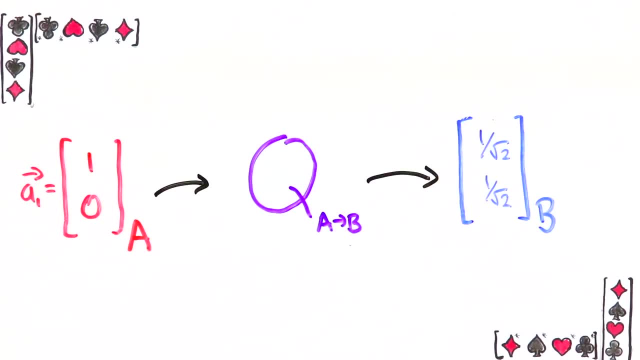 in Bob's basis. From this fact alone, and not from any calculations, work out what the first column of the change of basis matrix should be. Pause the video and give yourself a minute to think about it. If you weren't sure how to do this, I explain it in my video about matrices. 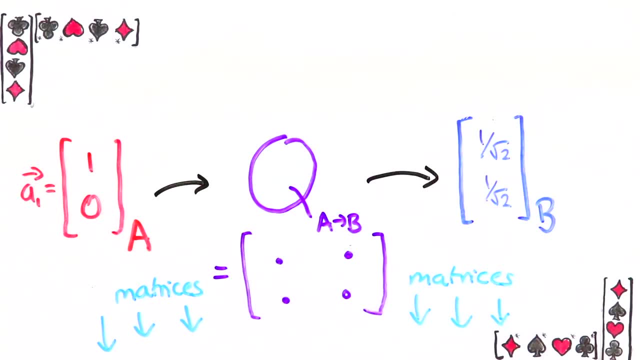 so go have a look at that in the description and my playlist linked in the corner. But remember the columns of a matrix just tell you what happens to the basis vectors. The first column is what happens to the first basis vector. here it becomes this: 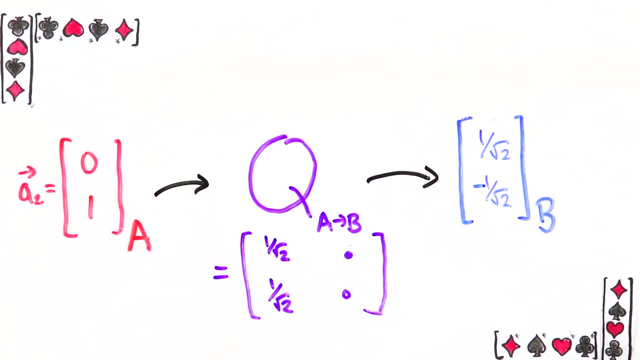 Similarly, the second basis vector becomes this: and so that's your second column. This is exactly the matrix we wanted, because if Alice puts in the column CD, it comes out as this column, just as we calculated earlier. but there's one really strange thing about the matrix. 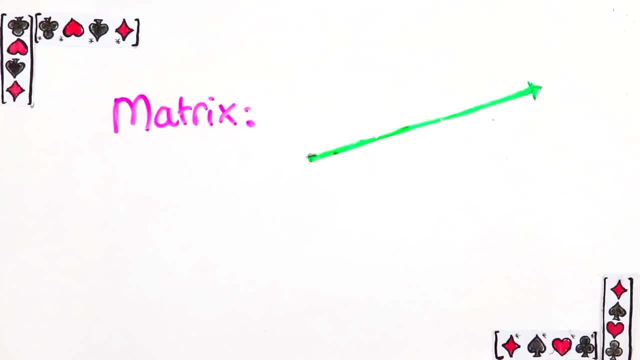 Usually a matrix takes a vector and transforms it to some other vector. That's not what's happening here. It should always be in the surface, because that'sGANラ SOize is переведка. this counts the distance between the matrix and the column, but there's no. 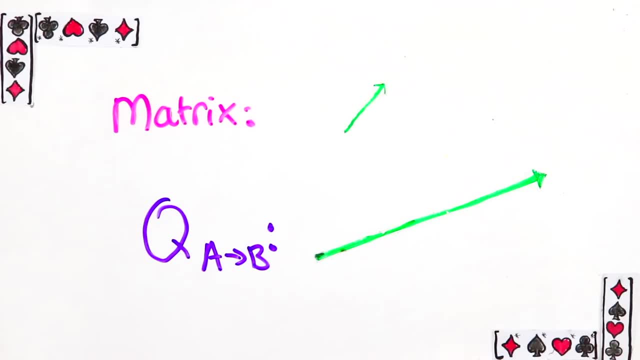 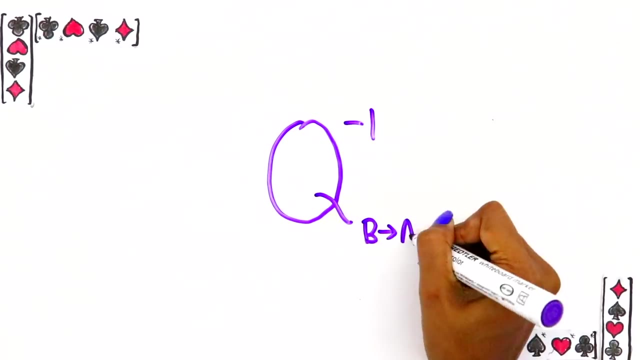 takes a vector and gives you back the exact same vector. it just changes how you describe it. That's something to keep in mind. but despite this, the change of basis matrix is very useful. For example, you can compute its inverse, which has an important property. 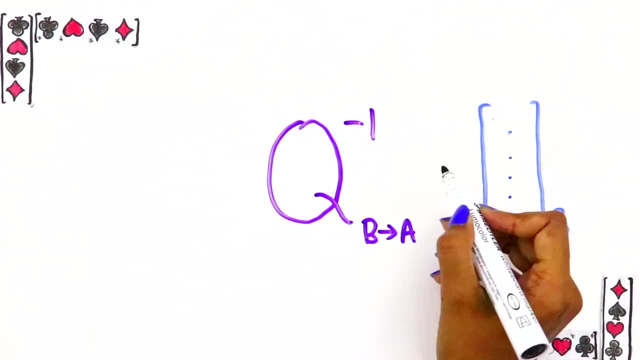 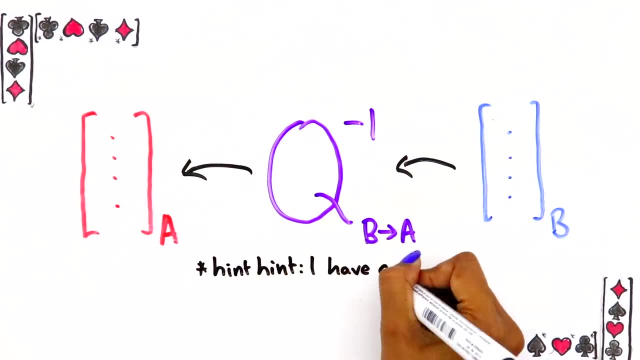 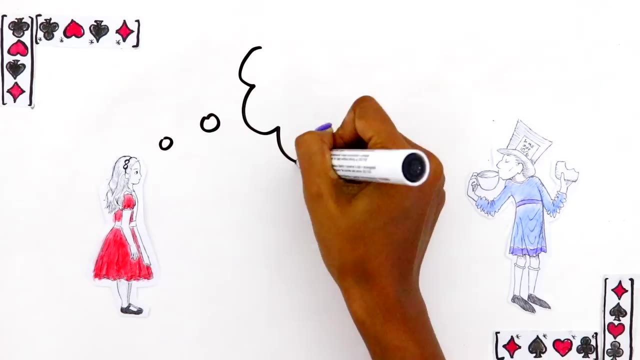 The inverse takes a vector that's in Bob's basis and translates it back to Alice's basis. That's just because that's what inverses do. They undo the original matrix. So once Alice has figured out what the change of basis matrix Q is, 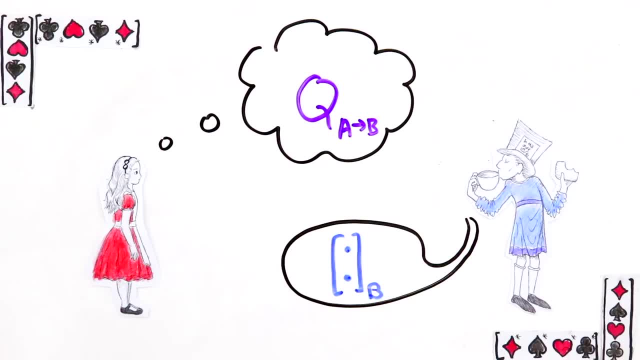 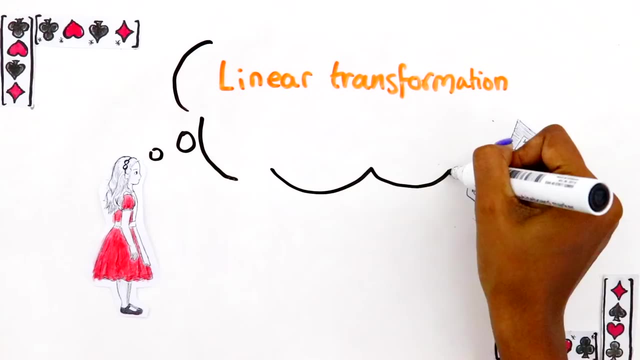 if she wants to translate a vector, Bob tells her to something she understands, she just applies Q inverse to it. There's another reason that these two matrices are super useful. If Alice now wants to describe a whole linear transformation to Bob, not just a vector, 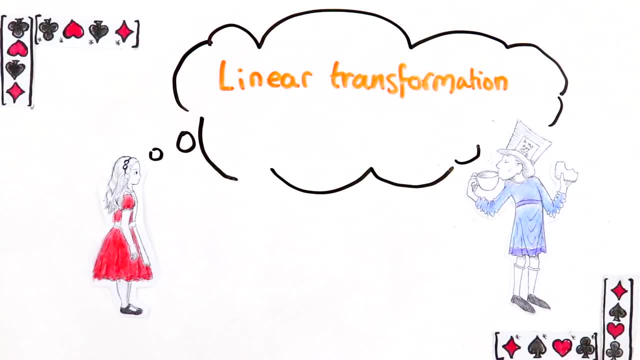 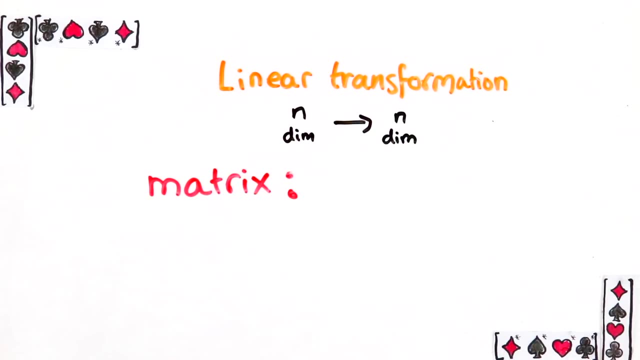 she can use Q and Q inverse to do it. Let's see how this works for the case when the linear transformation is from n dimensions to n dimensions. The easiest way to describe a linear transformation is to write it as a matrix, But the problem is the way the matrix looks. 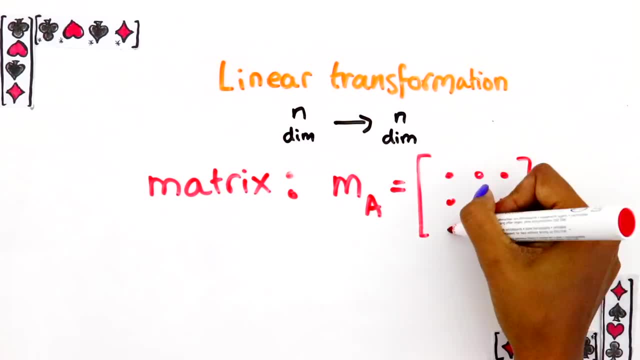 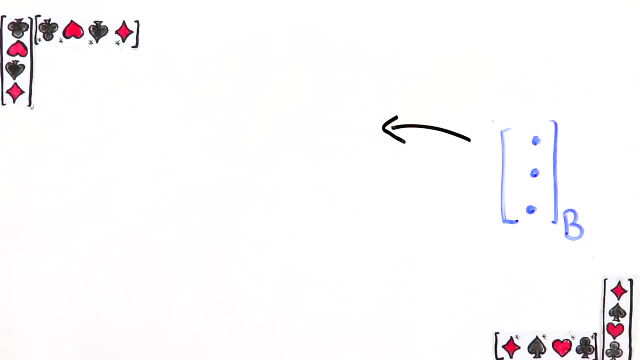 depends on what basis you've used. This is what hers looks like in her basis. Now she needs to translate it to Bob's basis, which means it will look very different from her own. Here's how She wants this matrix to take: a vector written in Bob's basis. 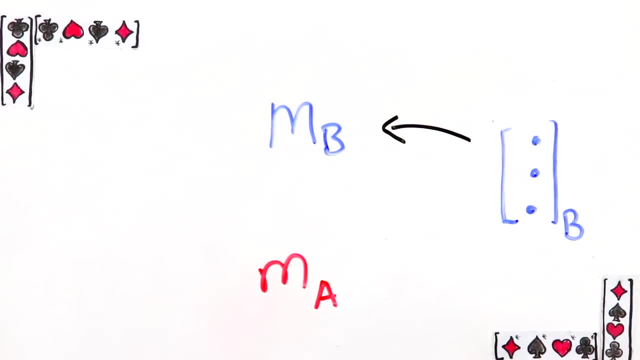 and do the linear transformation. But her current matrix only takes vectors written in her basis. So why don't we just translate Bob's vector by applying Q inverse? This writes Bob's vector in her basis and in this new form you can apply her matrix to it. 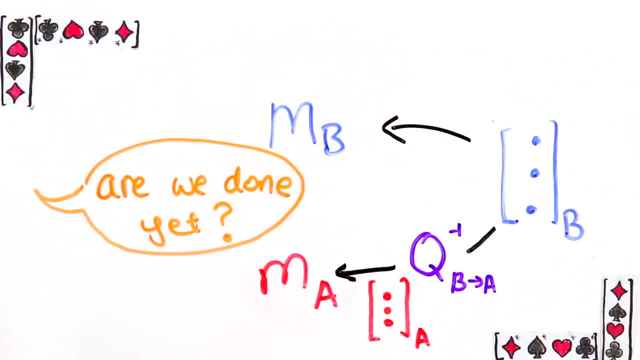 Okay, great, So are we done. Pause the video to think about whether this matrix M A- Q inverse is the matrix that she wants to translate. Pause the video to think about whether this matrix M A- Q inverse is the linear transformation we want in Bob's basis. 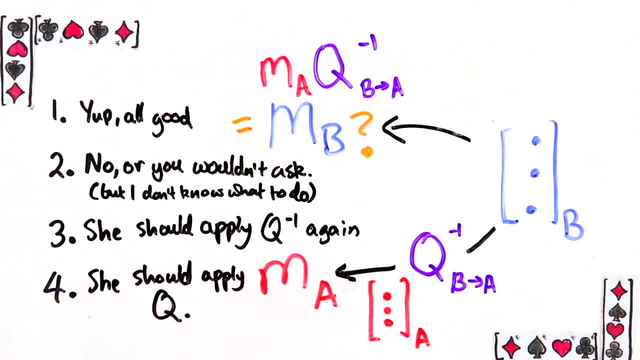 Then choose one of these options in the poll. One is yes, Two is no, but I don't know what to do next. Three is she should apply M inverse again. And four is she should apply M. Pause the video now and try and work it out. 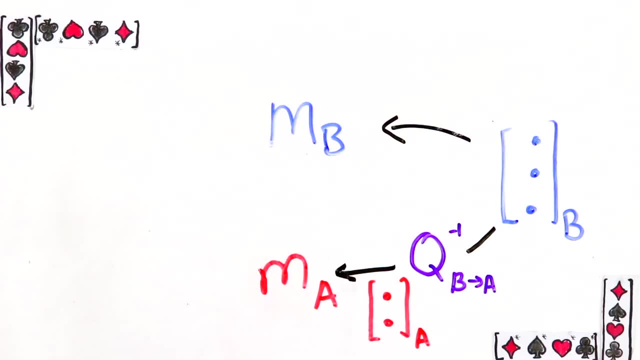 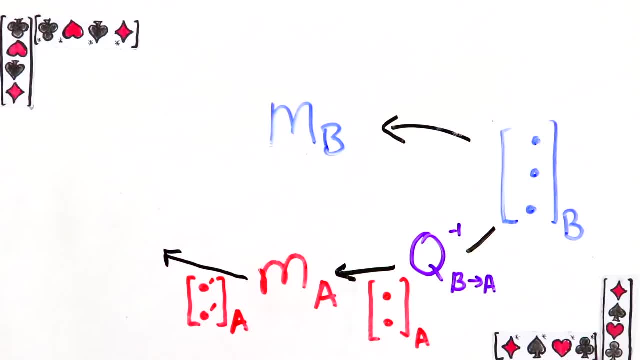 Because the column vector you end up with is not quite done. Because the column vector you end up with is not quite done. But that's no good, because Bob is expecting that his new matrix takes a vector written in his way to another vector also written in his basis. 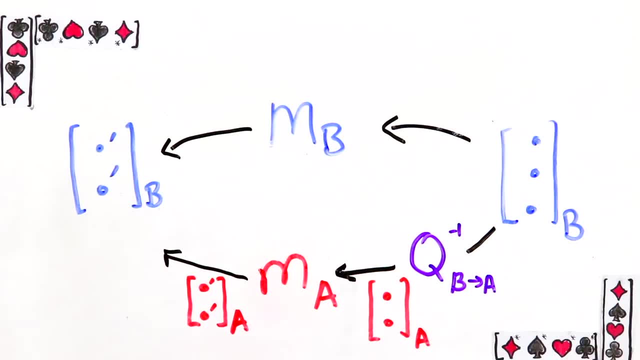 Unlike this, which is in Alice's basis. We have the right vector. it's just written in the wrong way, So we should apply Q to it and get it to Bob's basis, And now it's perfect. Overall, what happened is: 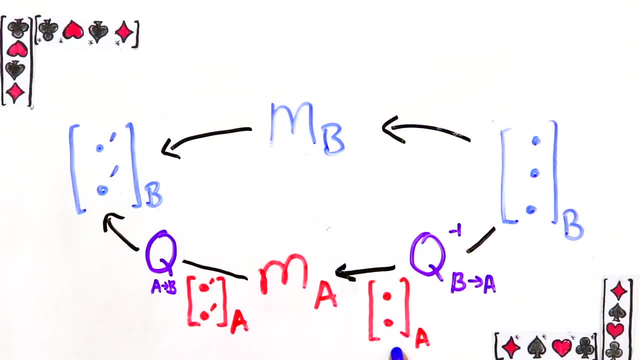 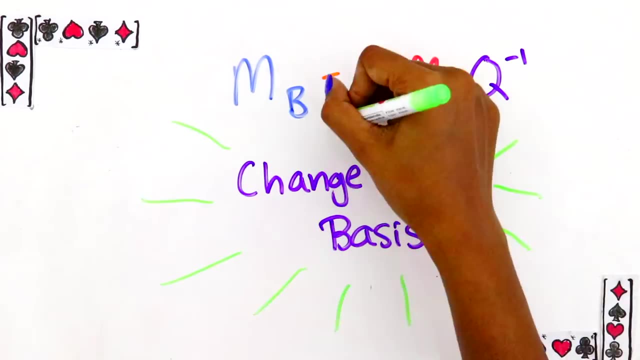 what happened is it got translated to Alice's basis. then you apply Alice's matrix, then you translate it back to Bob's basis. In other words, Bob's matrix is Q, M, A, Q inverse. It's a really simple concept when you understand it, but it's super important.